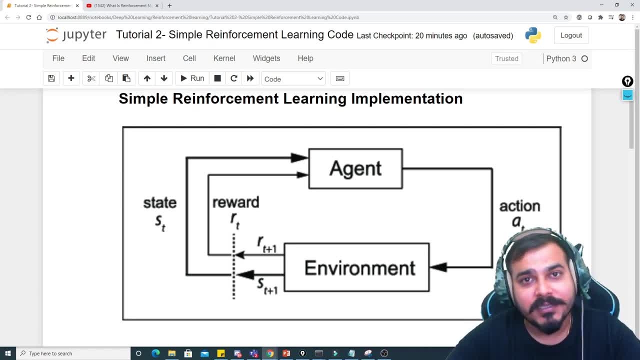 Hello all my name is Krishnayak and welcome to my YouTube channel. So, guys, we are into the second tutorial of reinforcement learning And in this particular video, we'll try to implement a simple reinforcement implementation where we'll just try to create a small application. it will be hardly, you know two to three classes. we'll just try to write a very basic code and see that how reinforcement learning can be implemented. Okay, If you don't know, as I said, this is my second tutorial. if you have not seen it, you can watch it. 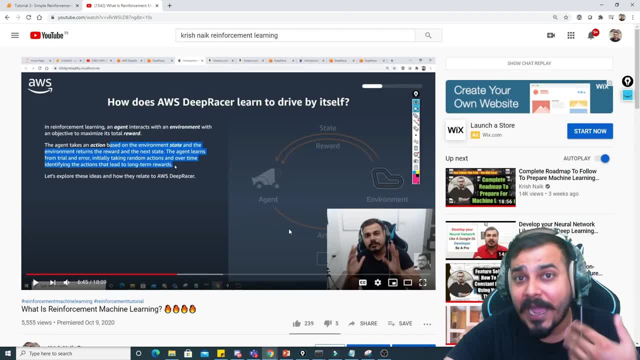 If you have not seen the first tutorial, this is what the first tutorial is: that where I've actually explained about what is reinforcement machine learning. And if you don't know about reinforcement machine learning, guys, as we know, in machine learning we have supervised, unsupervised, and reinforcement supervised and unsupervised. I have been uploading a lot of videos in my YouTube channel. Reinforcement learning is a complete, different section, So I've created a separate playlist for this. So please make sure that if you have not seen the first video, I'd suggest just go through this particular video Here I've taken 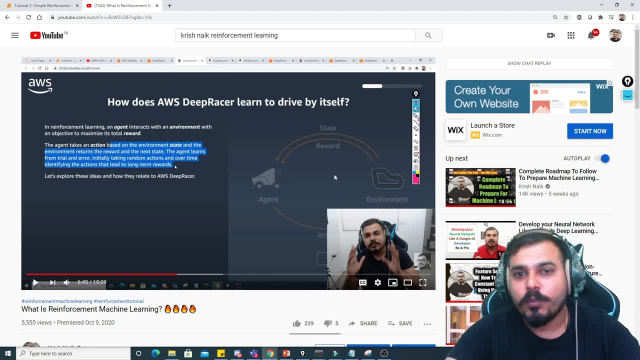 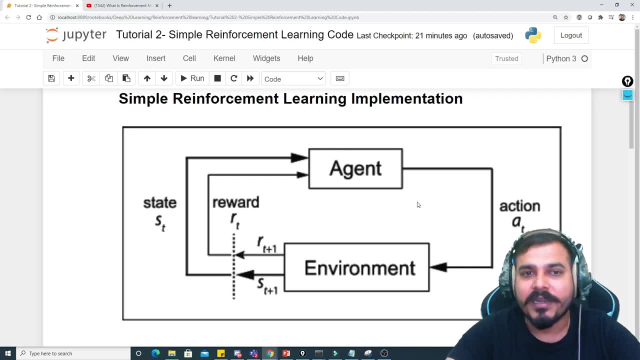 an example of AWS, but the implementation wise, the basic theoretical understanding has been clearly been made in this particular video. Now, in this video, we'll try to just implement a simple reinforcement learning application with the help of Python code. Okay, Before going ahead, guys, you need to really understand the smaller components of the reinforcement learning right. What are the important components? I'll not say smaller, but the most important components. that is agent, then you have 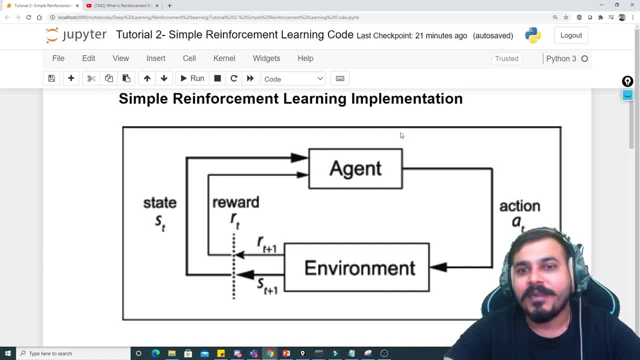 environment. Now, based on the environment, the agent takes a specific action And based on this particular action, the agent receives a reward. Okay, it may be a good reward, it may be a bad reward, And whenever the agent is receiving a reward, the state of that particular agent may also change. Now, considering this, we will just create a smaller Python application which will be able to learn in this specific way- I'll not say learning also, but at least. 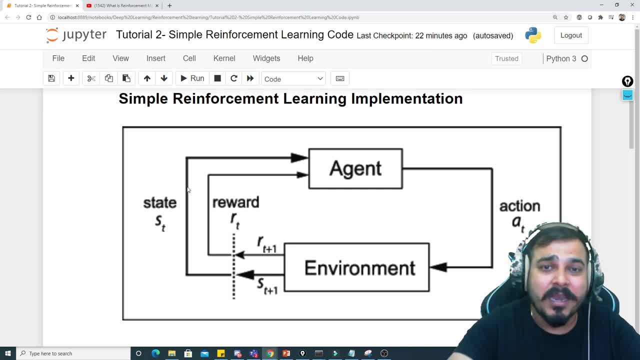 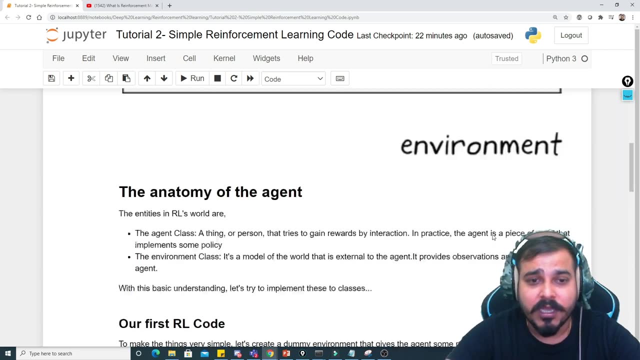 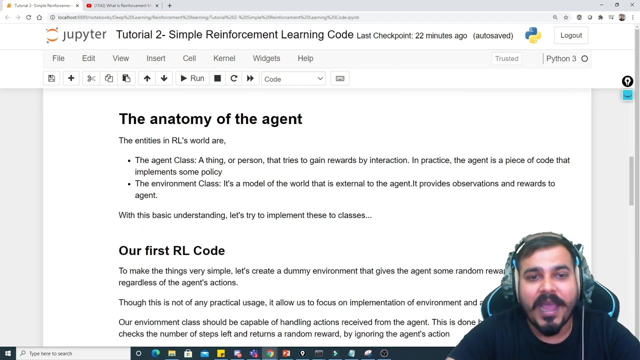 implement this part, where it is at least receiving a reward, a different kind of reward, a positive reward or a negative reward based on some specific action. That is what we'll try to create. We have a lot of frameworks in reinforcement learning, which I'll also be trying to upload in my future videos. Now let's go ahead. What is the anatomy of agents? So first of all, we'll discuss about this particular agent. Okay, What is the anatomy of the agent? You can see that the entities in RL world, that is the 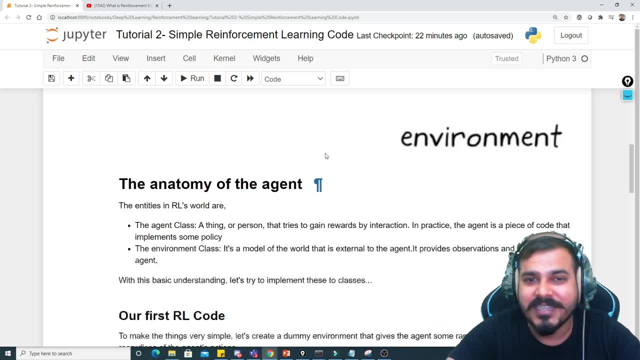 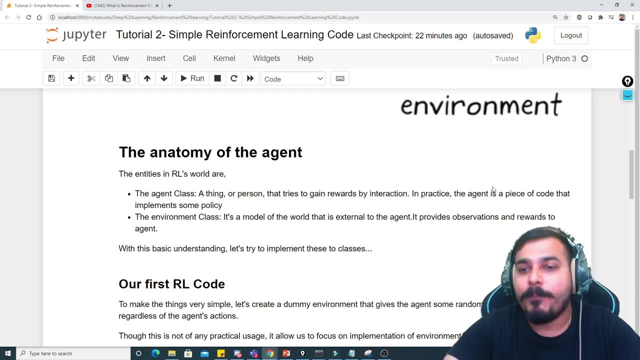 enforcement learning world are the agent class. What is this agent class? What is this agent class? It can be a thing or a person that tries to gain rewards by interaction. In practice, the agent is a piece of code that implements some policy. Okay, agent is nothing, but it is a piece of code which will be implementing some policy. I'll discuss about this policy, what it is, But you have to really remember this: what it is, it is just an entity. In short, you can say that agent class is just like an entity. 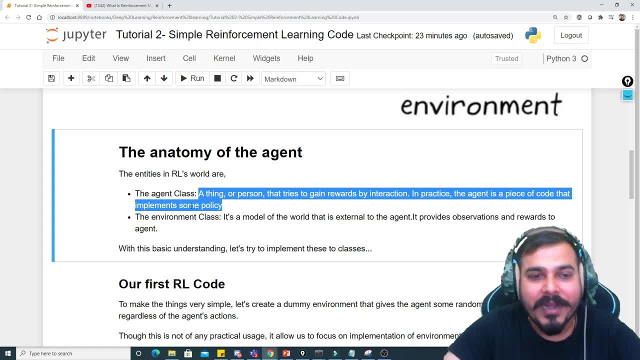 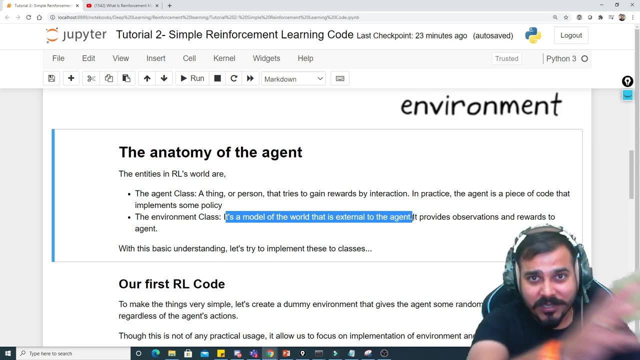 It is just like a piece of code that will be implementing some policy. Okay, the next thing after agent, The next thing we need to understand is about the environment class. now, the environment class, It is a model of the world that is external to the agent. Like suppose, if I am walking on the road, Right road is the environment, I am the agent. 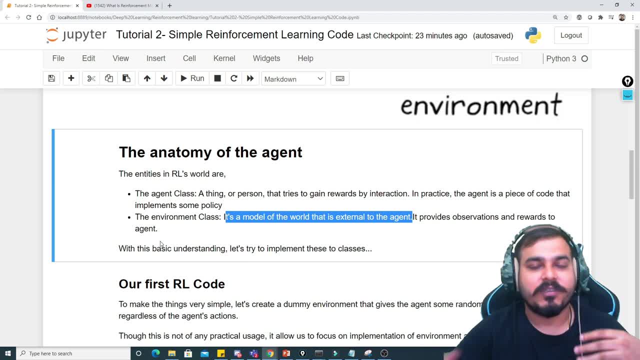 Okay, it provides observation and rewards to the agent. Suppose I am the agent, I am working in the road, suddenly there is a turn on the road- than obviously by seeing that particular environment it might be better I understand the agency here. 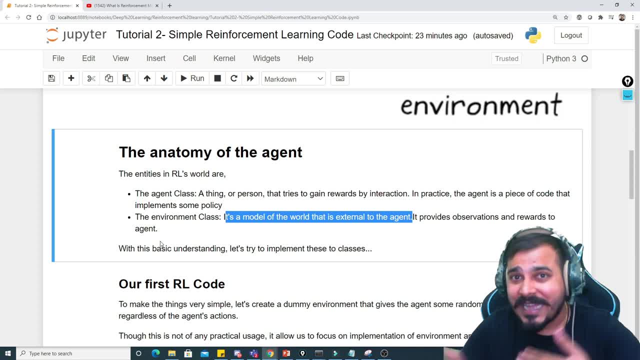 Okay, so the agent class. right now, it's everything you have to know about the agent class. Let's see how this agent class works. Okay, so that helps us understand. i will take a turn in that specific road. right, so that is how a agent also learns. and if i'm 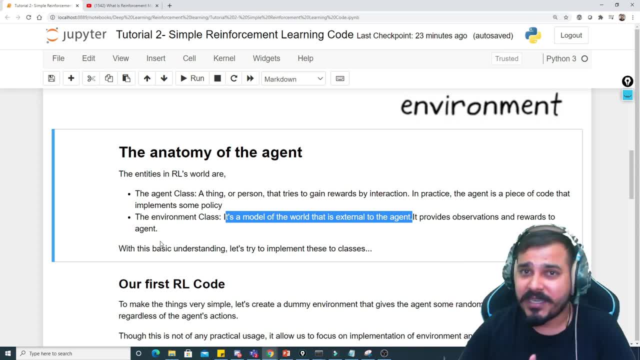 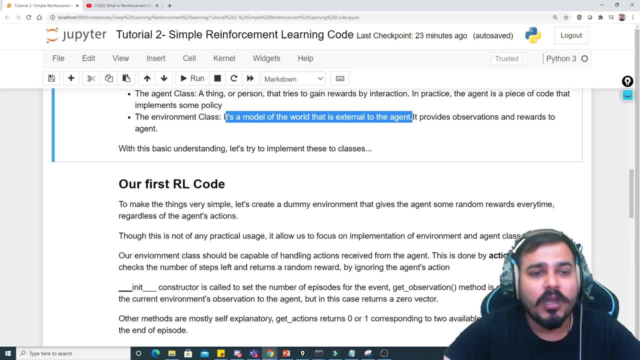 turning in the right position, i'll be able to reach my destination very, very quickly, right, and that is how, in the reinforcement learning also, similarly, the agent will learn. okay, so let's write our first rl code. okay, now, first of all, what we'll do is that we'll try to create a class. 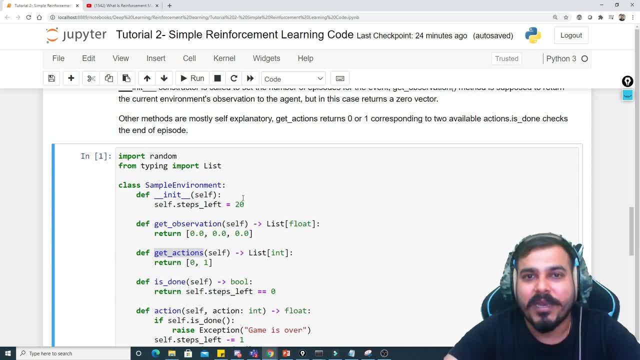 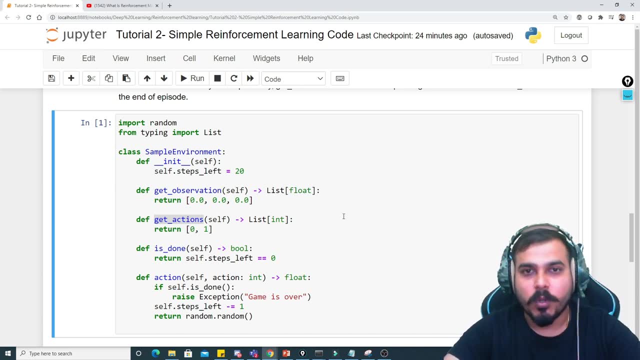 environment. so here we have created a class sample environment. and remember, guys, this is just basic python code. reinforcement learning is more about python code, guys, just simple implementation. we just need to find out the way that, how we can train the agent, how we can get, how we can capture. 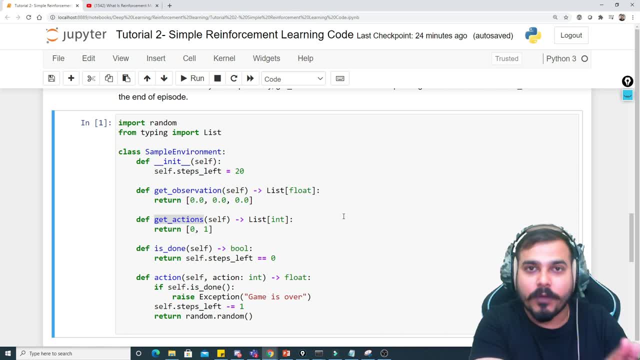 the new environment right and, based on that, what kind of reward we can actually provide it to the agent itself. so here we have created a simple class which is called a sample environment, and inside this we have a constructor which is called as init. okay, now this constructor. 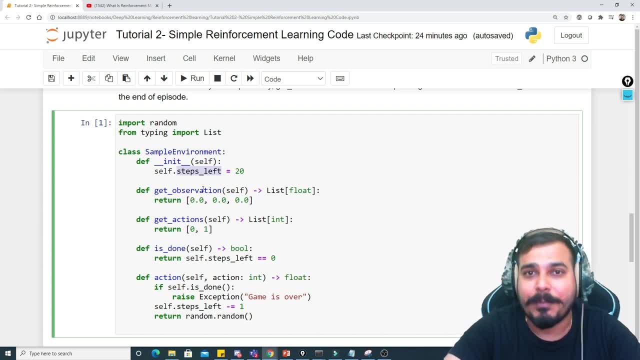 it is defining you a variable which is called as steps. underscore left is equal to 20.. this basically says that, probably, suppose, if i'm designing a game and it needs to be completed in 20 steps, so that is what i have actually kept over here. just think in that specific way. okay, in this problem statement i've 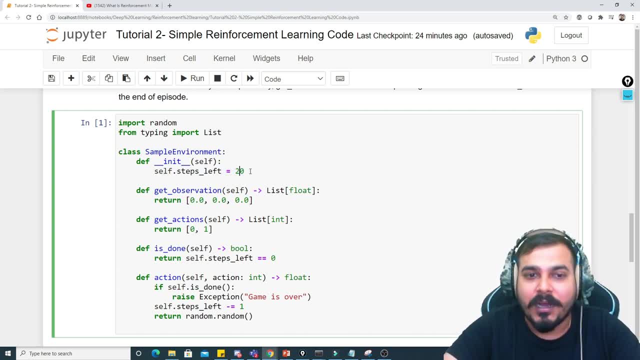 actually kept a variable which is called as steps, underscore left, uh, which is just like 20 value. this is like the maximum number of steps in this the agent can take, agent can basically take in order to gain the rewards. okay, you can think in that specific way. the next thing is that here you have a function which is called, as we have defined, a function inside this environment which is called as get observation, observation, observation, okay, and this. you will be getting some three coordinates, and this can be any kind of coordinates, guys, not only three, you may also be getting four, you may be getting five, you may be getting six, anything right. so this information is nothing but the information regarding the environment. okay, here i have just defined a function inside this environment which is called as get observation. okay, and this. you will be getting some three coordinates, and this can be any kind of coordinates, guys, not only three, you may also be getting four, you may be getting five, you may be getting six, anything right. so this information is nothing but the information regarding the environment. okay, here i have just defined a function inside this environment which is called as get observation, observation, observation, okay, and this. you will be getting some three coordinates- and this can be any kind of coordinates, guys, not only three, you may also be getting four, you may be getting five, you may be getting six, anything right. so this information is. 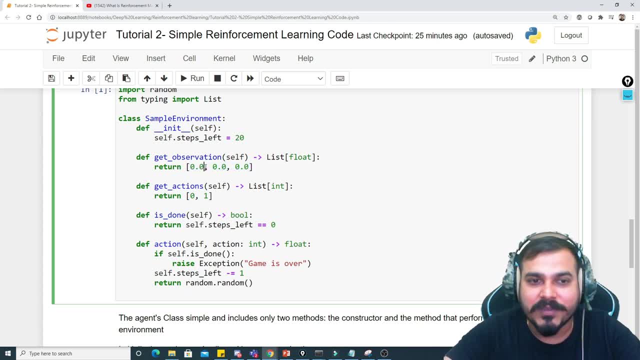 randomly written it as three by just placing some values like 0.0, 0.0 by 0.0. we have still not decided, and probably i'll not be implementing in this video, like: how do we decide? you know what the environment value should get returned? don't worry about this, this can be anything. okay, this may be some kind of logic which is actually giving you some information regarding the environment that you need to understand here. i've just hardcoded it to 0.0, 0.0 and 0.0. 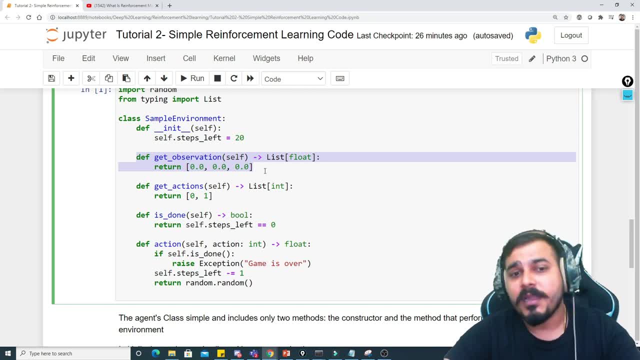 that is the main thing that you need to understand now. the next step is basically get actions. now, this guest action is nothing but by when the agent performs a specific action, he or she should be getting some rewards right, and that rewards may be one or zero. in this particular case, i'm giving one and zero. the reason why i'm giving one is zero. i'm considering one as a positive reward. i'm considering zero as a negative reward. okay, so re. 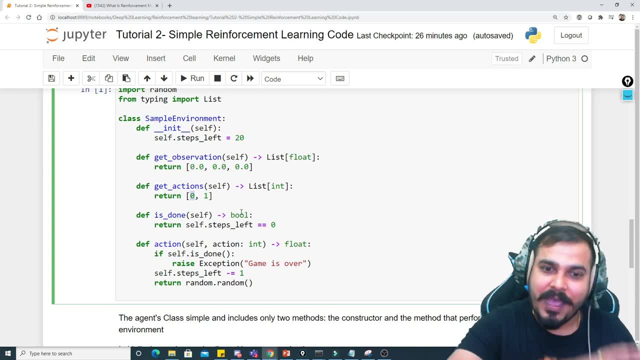 the agent over here will be performing some action and based on that they will be getting some kind of rewards. so for that we have defined zero and one. what are the possible number of? uh, that basically means what we are going to do in this particular code. i'll just show you. but in this get actions it is giving two rewards: zero and one. okay, zero and one every time. in this get observation it is giving three values. all the three values are zero. i have just hardcoded it, the logic. the logic has not yet been written because this is a simple rl. 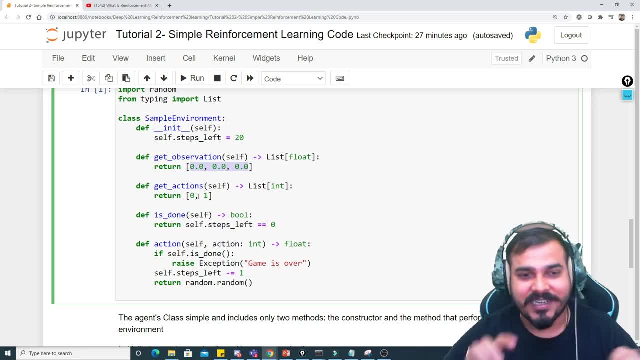 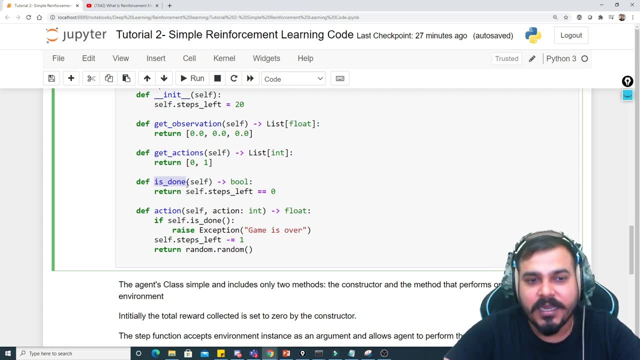 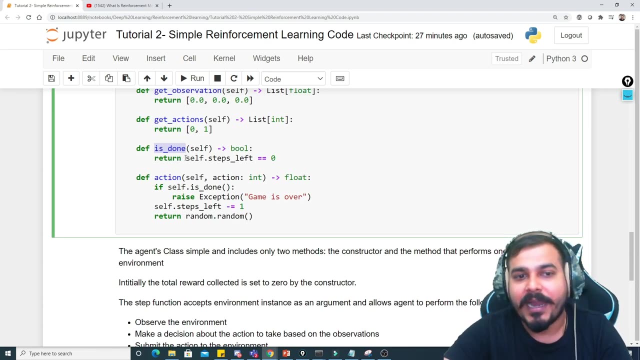 code implementation. okay, so logic, we have still not decided. logic will decide in the upcoming videos. then there is also another function which is called as is done is done basically means when your the step left will get completed. at that time we will try to send a boolean value from this function. suppose if the steps has been completed, we should basically say some boolean value saying that yes, the steps has been completed. this will give an. 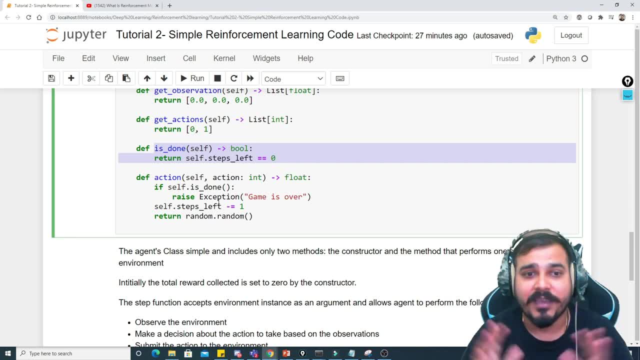 indication that now the agent will not be able, should not be moving here and there. okay, finally, this is basically the action step in the action step. first of all, whether the agent should take an action or not, how it'll check. first it will call this particular function. it will go and see whether the step step is. is there any step left? if 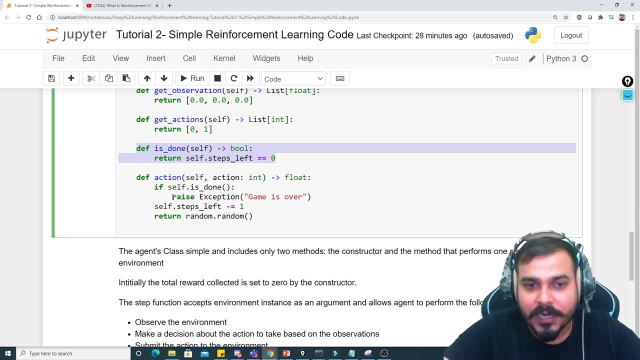 it is not left. if it is not left, then only it raise a exception saying that the game is over. if it is left, it is just going to decrement that particular step. okay, and then it is returning some random value. okay, this is just a simple implementation. now, this was with. 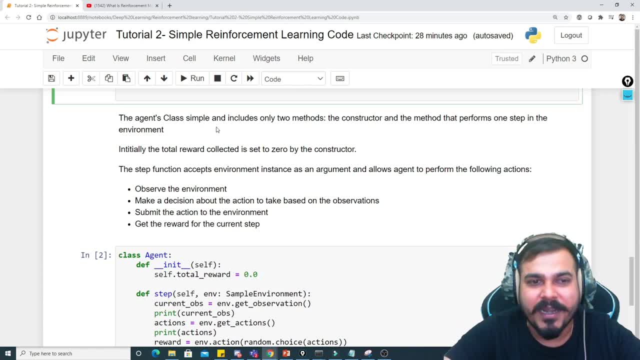 respect to your environment, the same thing. i've explained it over here. okay, so you can see that the step functions. accept environment instances as an argument and allows agent to perform the following actions: observe the environment. make a decision about the action to take based on the observation. submit the action to the environment. get the reward for the current step. okay, now one. 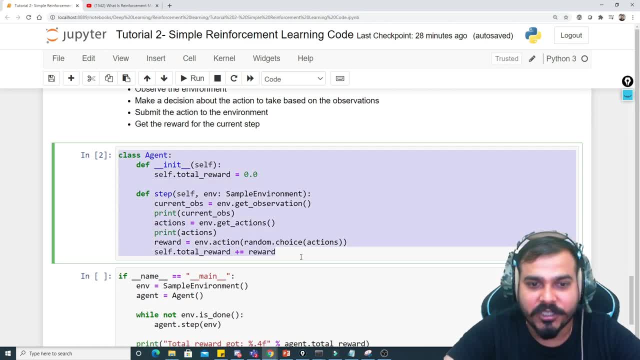 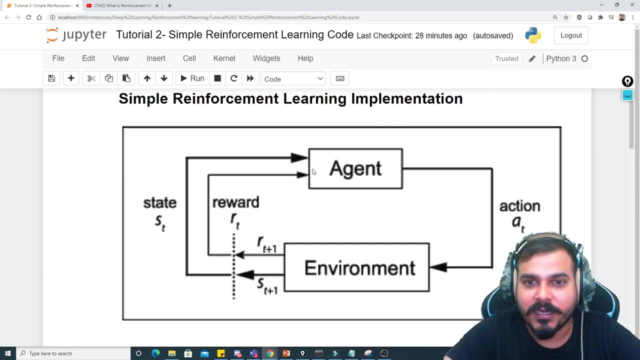 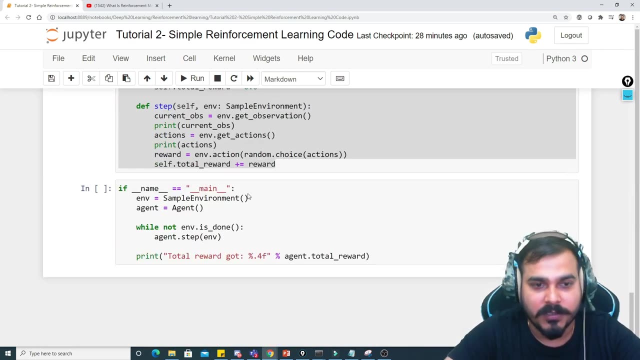 more thing i really want to specify, basically about the class agent. now, you, we have seen about the class environment. right, we have defined about this class environment and we have covered almost everything now with respect to the agent. agent will definitely be performing some kind of, will be implementing some policy. now what is this policy? okay, so here you can see, in agent we have 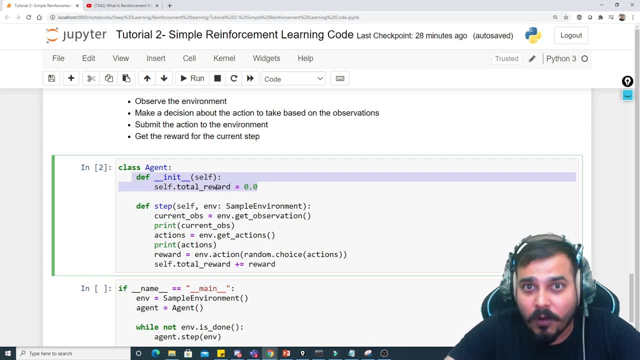 defined initially, the agent, the. the rewards that is basically been assigned is 0.0. okay, now the agent will be doing some, uh, it will be taking some movement based on the environment. it will be doing some kind of task based on the environment. so you can see that, observe the environment first of all. it. 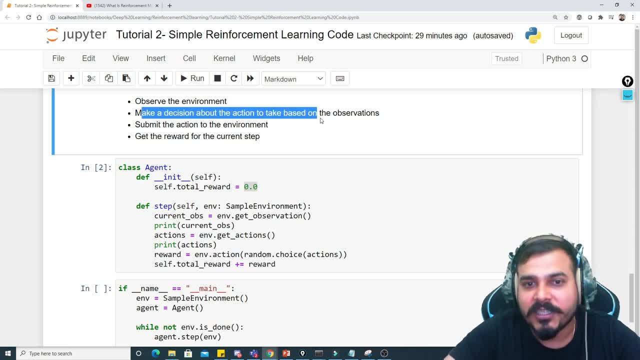 will observe the environment, then it will make a decision about the action to take based on the observation, and then submit the action to the environment and then he will be getting the reward. okay. so similarly, we will be defining over here. this is my function, that is, step over. here we are. 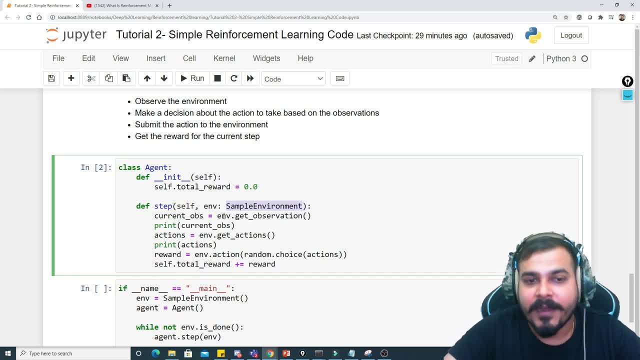 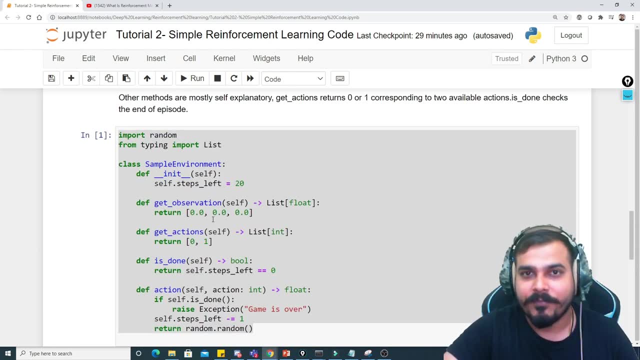 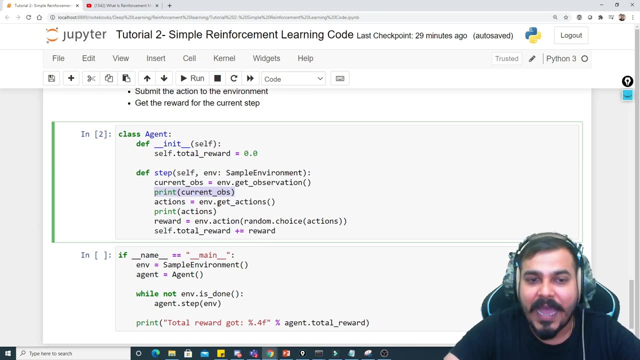 going to take the sample environment object. then we will get the observation. okay, this particular observation, how we are getting it, don't worry about it over here. we have just hardcoded it right. so we i'm calling the get observation here you'll be getting zero, zero, zero. you can see that i'm also printing this. then i'm getting the actions. 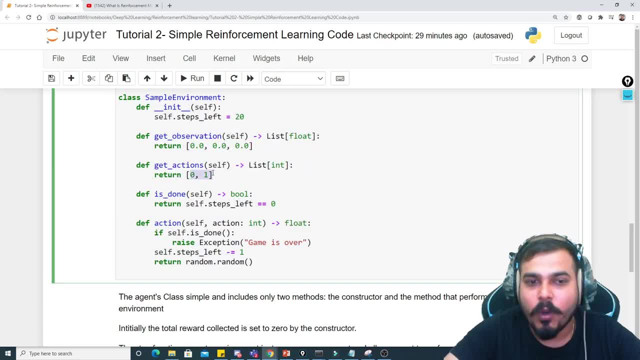 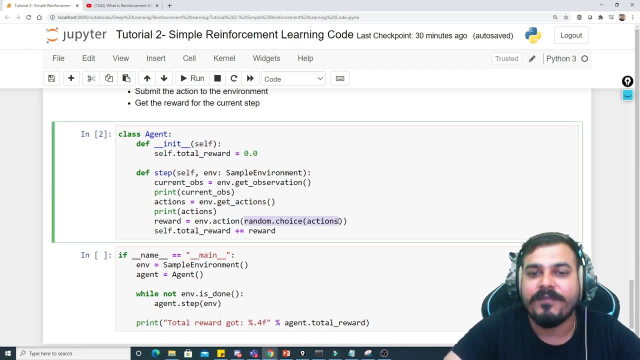 in actions. what are the values that you will be getting? you will get zero and one. right, you'll be getting zero and one. once you get zero and one, what i'm doing is that i'm picking up that action value randomly as a choice. i can either pick zero or one. 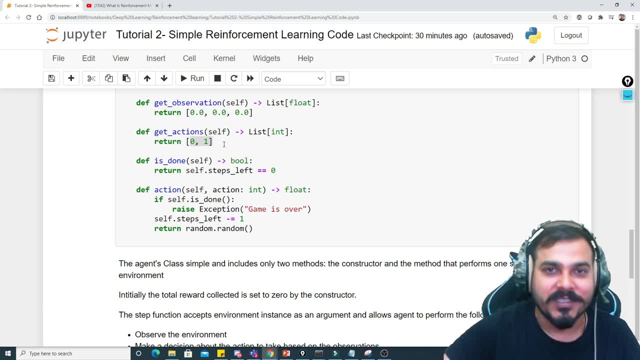 if i pick one, that basically says that it is getting a positive reward. if i pick zero, that is basically like it is getting a negative word. but why i am picking, that is not. i have not defined that whole implementation. i'm just randomly picking over here what kind of reward i should. 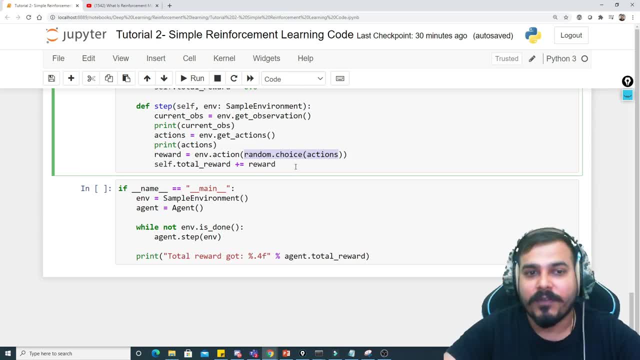 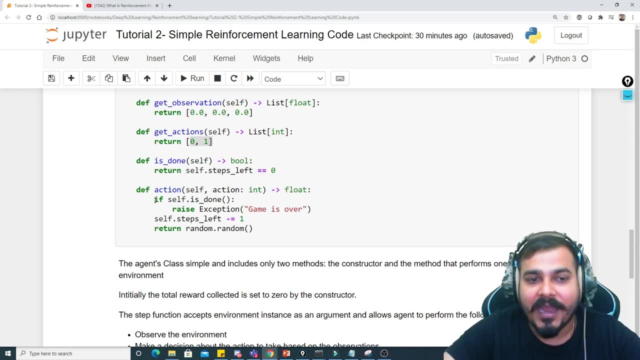 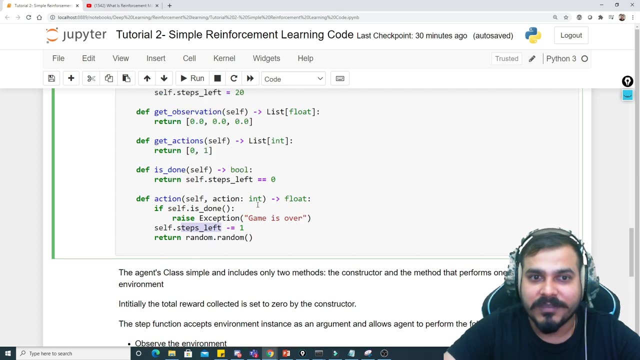 be giving this particular variable. okay, what kind of reward? okay, so here we can see that when we write envaction, it is, in short, calling this particular action over here, and then it will implement this. after implementing this, it will say that it is getting a positive reward. okay, so we will try to reduce this particular step by one, because 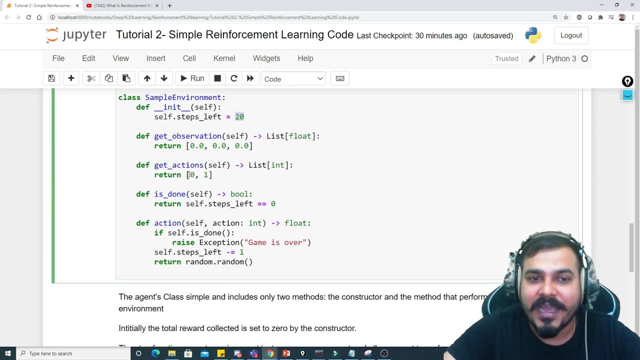 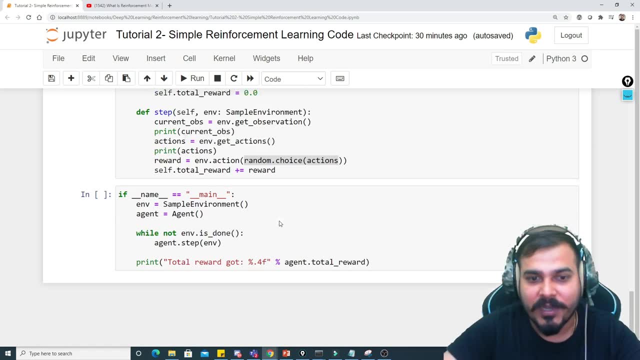 we know that the maximum number steps are 20, so we'll try to reduce this step by one every time we are calling this and then we will be getting this particular value, only one of the value, not both. the value it can be randomly picked. right now, again, i'm telling you guys, here we have not. 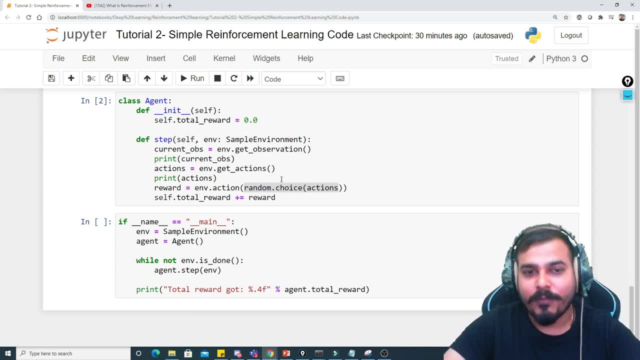 written. any logical logic is just like we are randomly picking up the rewards, right? usually what happens is that when i call this, get action, or when i call this action, there will be some positive rewards. okay, so we will be getting the negative rewards if that path, if the, if the, if the, 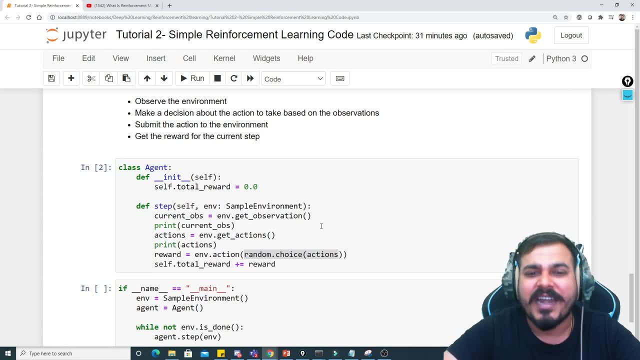 decision of the agent is correct, then only we should be providing the positive rewards, okay, otherwise you'll be getting the negative rewards. here we have just randomly taken this, so finally we'll get that particular word and finally we'll be adding the reward after we call this agent. 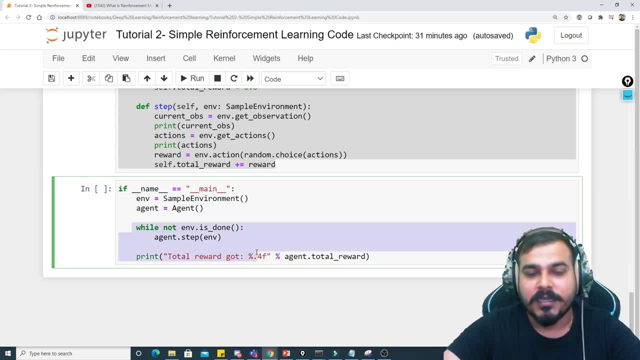 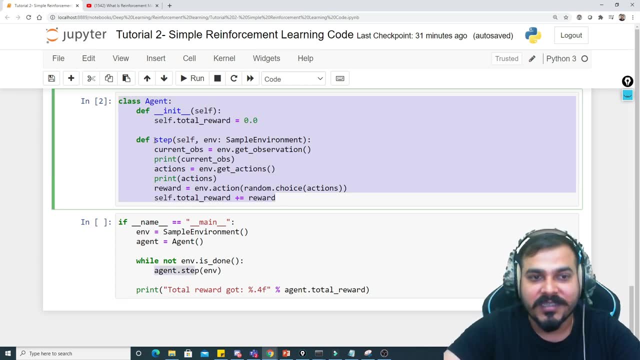 functions. you'll be able to see in this right, when i'm calling, first of all i'm calling environment, i'm calling agent and then i'm calling this. we are calling this agent dot step. this agent dot step is nothing but this function and this, in turn, will be calling all these particular functions, right? so like this for. 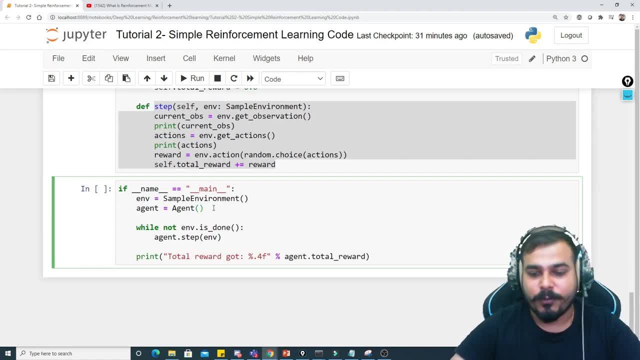 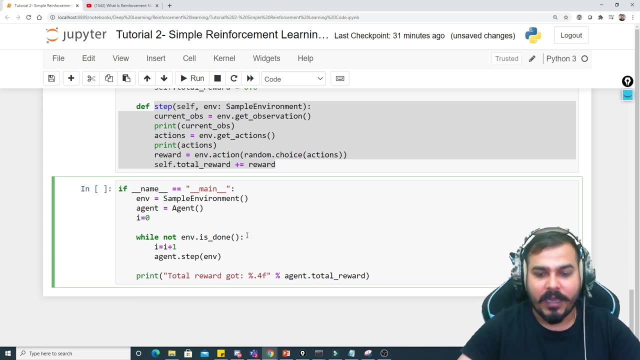 how many number of steps it will happen. let's see how many number of steps. suppose, if i start over here, i'll say i is equal to zero, okay, and then every time i will increment: i is equal to i plus one, and then i'll print i okay, i'll say that, okay, this is my steps. uh, steps, uh, with some value, okay. 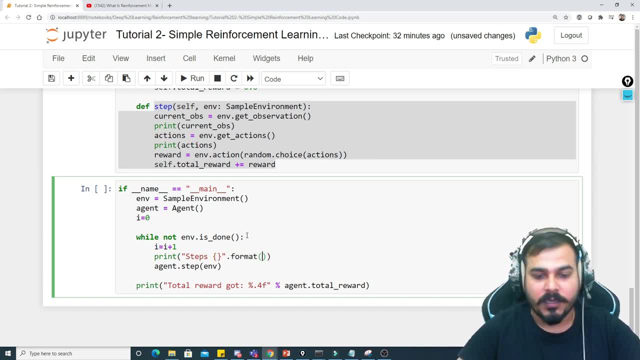 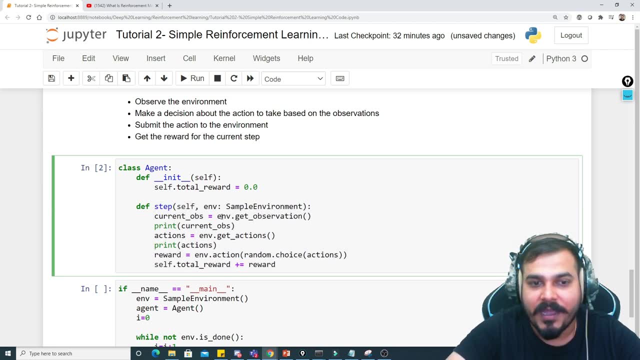 and then i'll write dot format okay, and here i'll write like this. so it will say: step one after step one, what will happen? we'll call this function, this function is calling this one right, and inside this we'll get the observation and we are printing the observation. see, 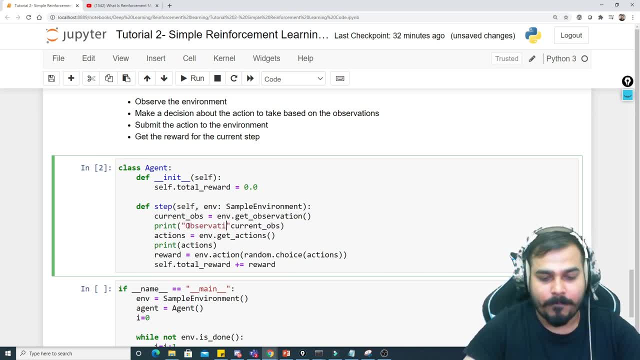 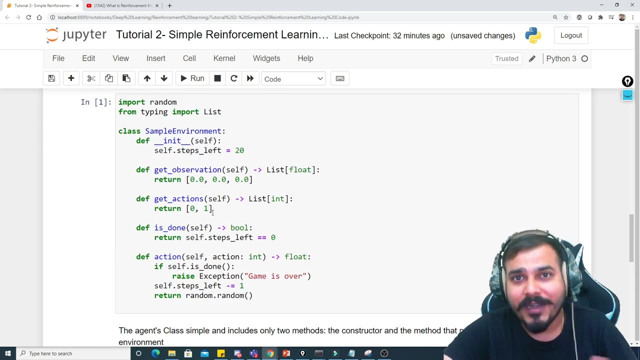 i'll print over here the observation, observation, right, and this will be zero. only because i have not written any format, right? this will always be zero. i cannot change that. what will be the action? the action will also be like 0 and one, because here we have not written the whole logic, right? this is just that we want to train it. 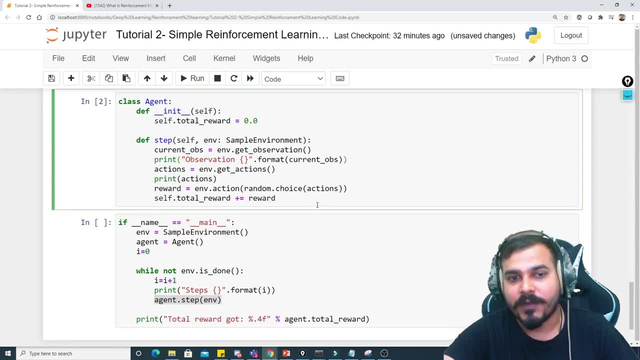 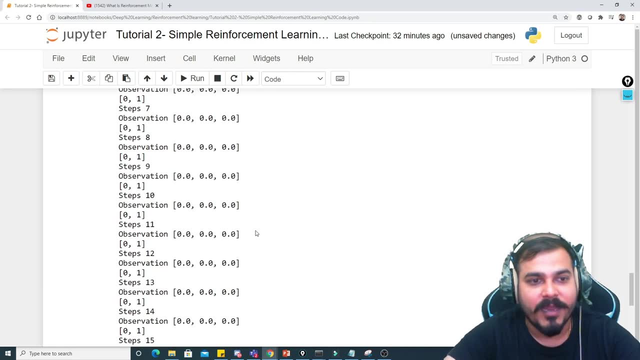 for 20 steps and it should be able to get maximum number of rewards. okay, and then you will be able to see: we have done this, we have done this, so let me just execute this. let me just execute this now. here you'll be able to see guys. see, in the step one the observation is written this: this: 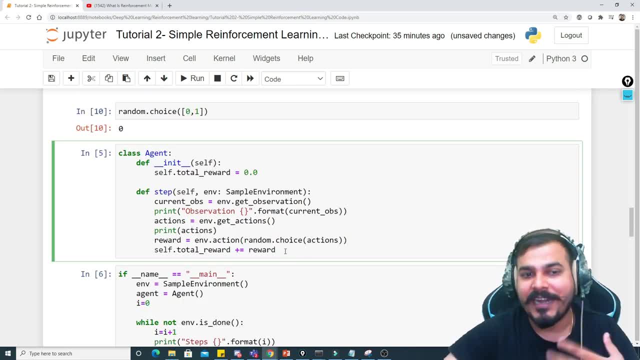 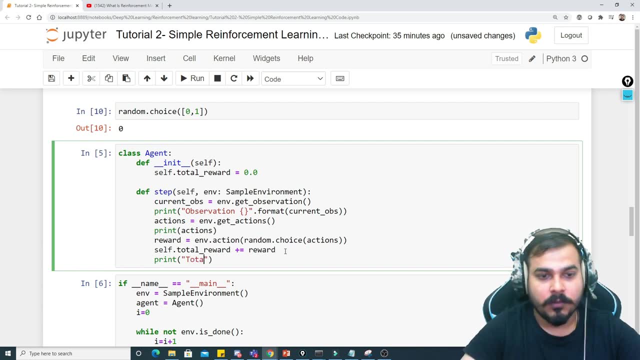 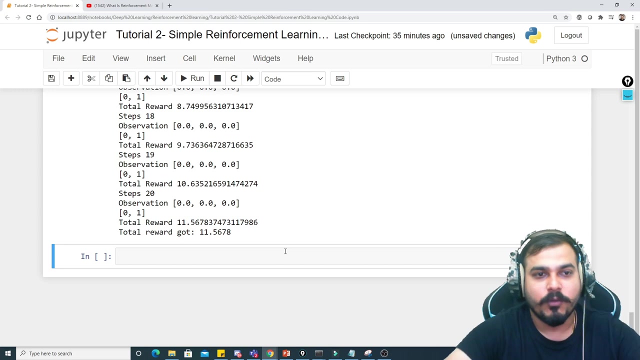 okay, we'll also try to calculate the total reward and we'll try to print the total reward every time let's see. so here i will say that my okay, total reward okay is nothing but by a placeholder dot format okay. and i'll say: self dot: total reward okay. so after every iteration i'm probably trying. 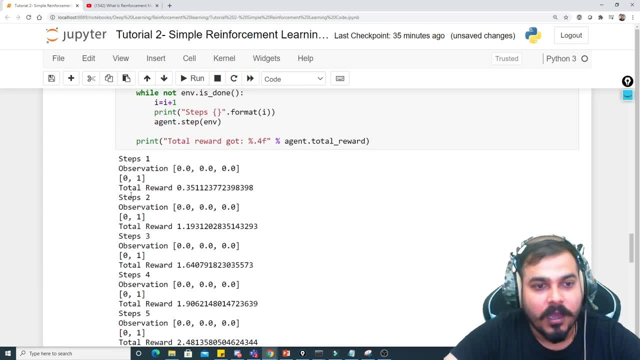 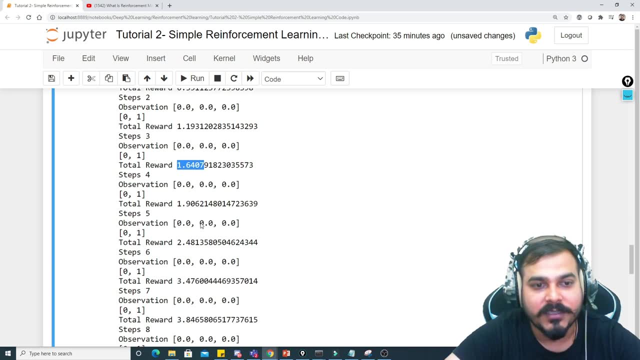 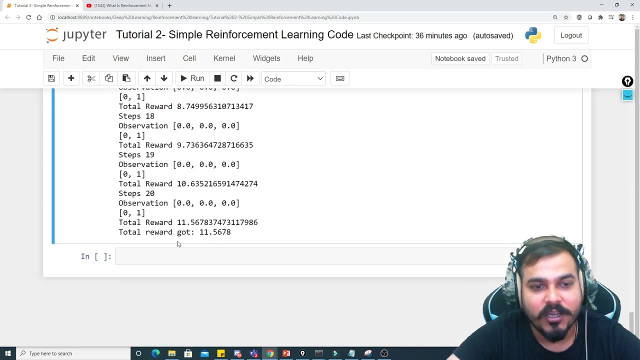 to print it. okay, now here you'll be able to see guys see: uh, the total reward over here is 0.351. then it became total reward 1.193. after step 3 it became 1.64, 0.906, 2.481, 3.46, 3.84, like this. finally, you'll be able to see that the total reward that we got is: 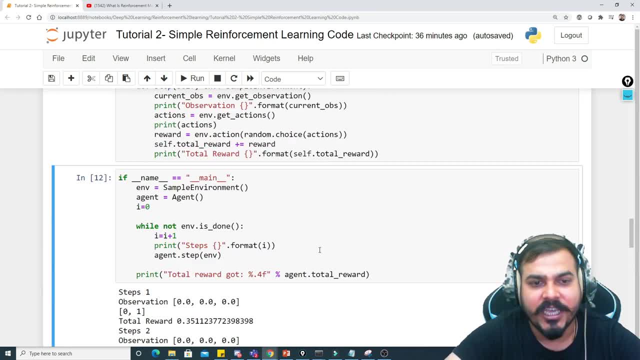 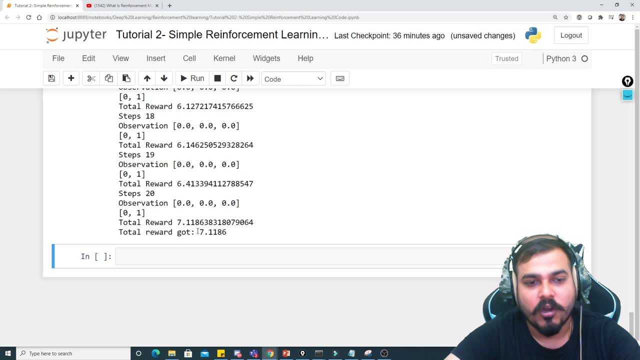 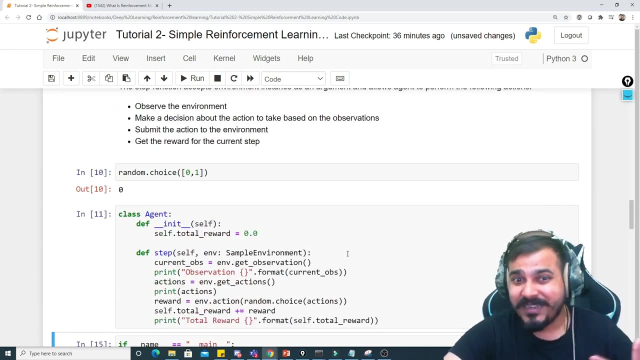 11.567 and every time, every time, it will change. every time, whenever i execute this, it will change. now, this time i got 10.7. okay, let me just execute it once again. then this time i got 7.1186. okay, then this time i got 8.28 again. we are running it for 20 different steps. right, and obviously our 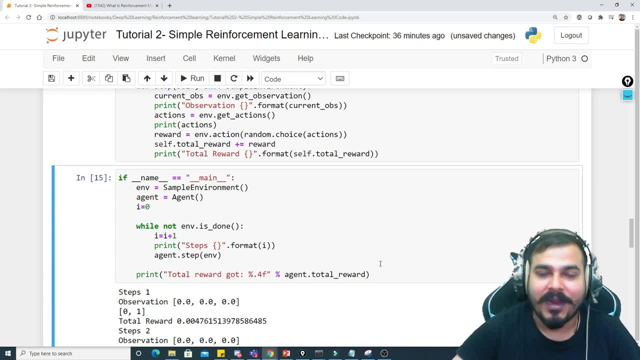 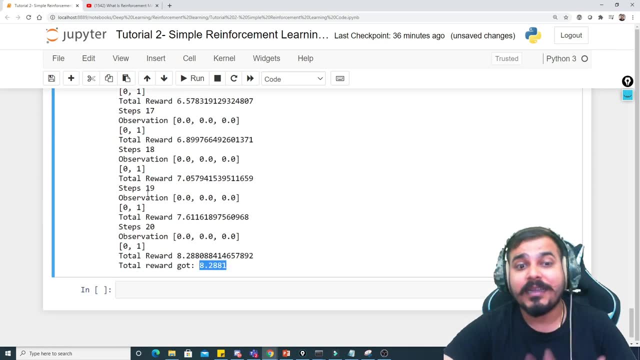 application should be running it for 20 different steps- right. and obviously our application should be running it for 20 different steps- right. and obviously our application should be trying to move towards that part from where it will be able to get the maximum reward. but here that all things are not happening, but at least we are accumulating the rewards. 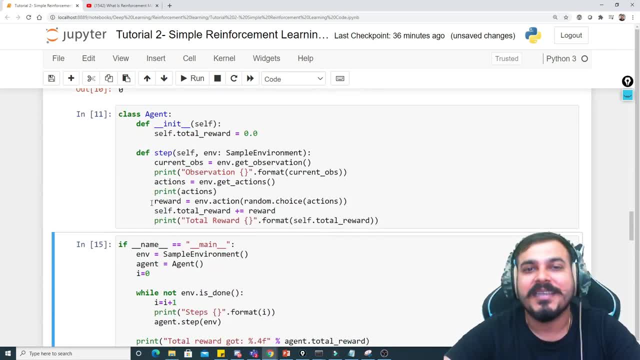 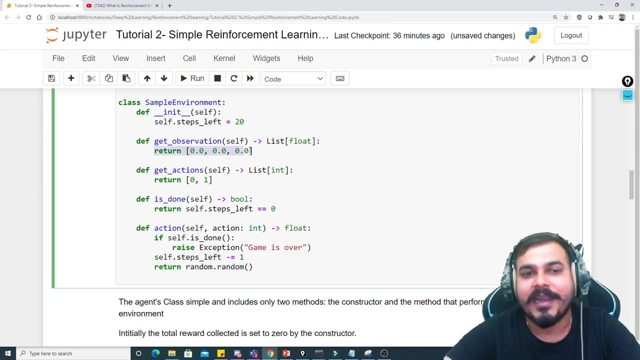 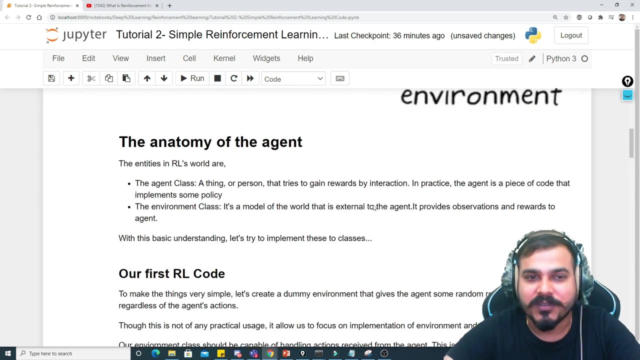 based on the environment. so i am saying you that this is the basic rl implementation code. in the upcoming videos, we will be seeing various frameworks like: how will we decide that, how to get this observation, how should we decide to give the rewards or not? all those things will be implemented in the upcoming videos, guys, but this is just an.